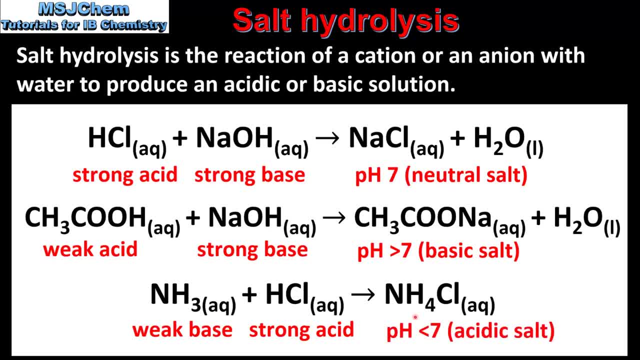 And in the last reaction, which involves a weak base and a strong acid, the solution formed has a pH of less than 7.. So these two reactions involve salt hydrolysis. This is where a cation or an anion from the salt 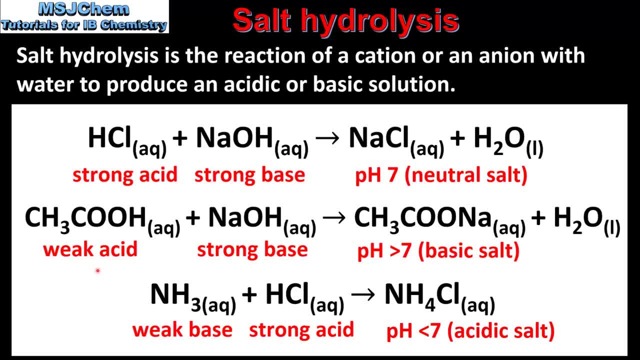 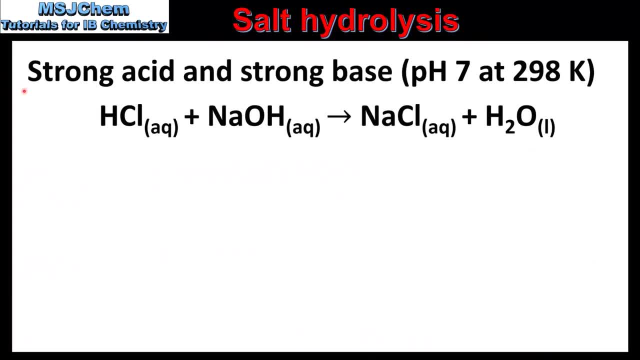 reacts with water to produce an acidic or basic solution. So next we'll look at each of these reactions in more detail. So we'll start by looking at the reaction between a strong acid and a strong base. So in this reaction, hydrochloric acid reacts with sodium hydroxide. 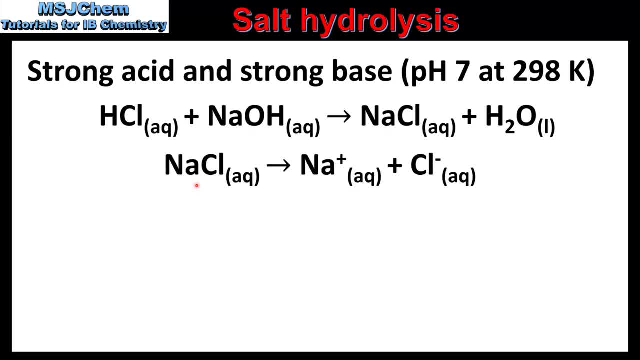 to produce sodium chloride and water. The sodium chloride dissociates to form sodium ions and chloride ions. Due to the fact that strong acids and bases dissociate completely, neither ion is able to hydrolyze water. Therefore, the solution formed will have a pH of 7 at 298K. 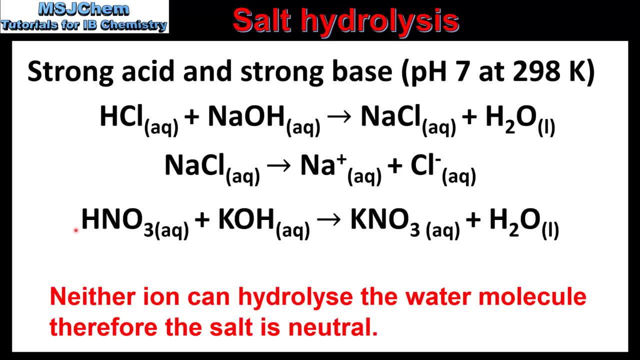 Another example is the reaction between nitric acid and potassium hydroxide. They react together to form the salt potassium nitrate. Potassium nitrate dissociates to form potassium ions and nitrate ions. Neither ion is able to hydrolyze water. 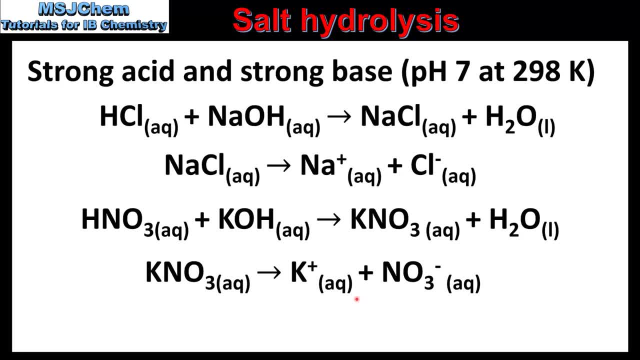 So the solution formed will have a pH of 7 at 298K. So, to summarize, the salt formed by the reaction of a strong acid and a strong base is a neutral salt. Next we look at the reaction between a weak acid and a strong base. 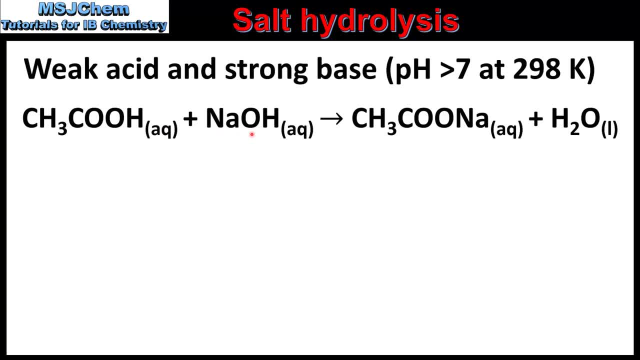 So here we have the reaction between ethanoic acid and sodium hydroxide to produce sodium ethylene. Sodium ethylene dissociates to form ethanoate ions and sodium ions. Sodium ethylene dissociates to form ethanoate ions and sodium ions. 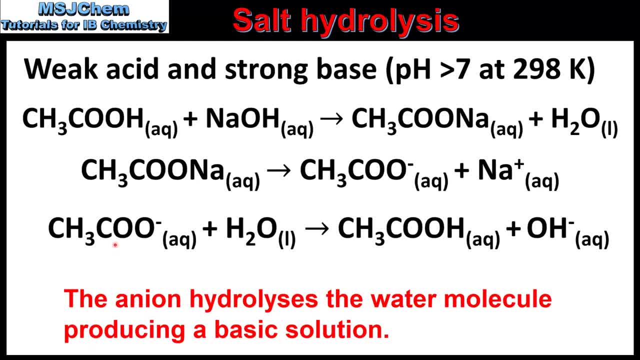 The ethanoate ion is the conjugate base of a weak acid. Therefore, it is strong enough to hydrolyze water. This results in the formation of ethanoic acid and hydroxide ions. Due to the presence of excess hydroxide ions, the pH is greater than 7.. 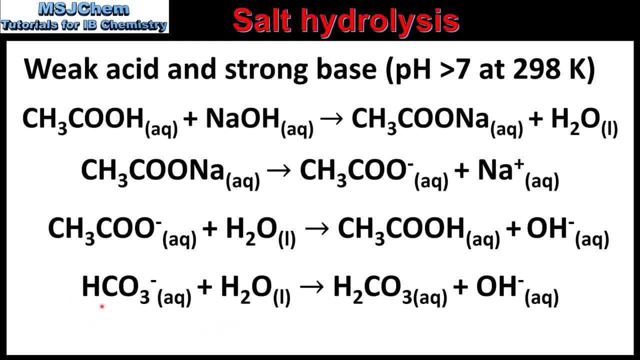 Another example is the reaction of the hydrogen carbonate ion, Which is the conjugate base of carbonic acid. This ion is able to hydrolyze water to produce carbonic acid and hydroxide ions. Once again, due to the presence of excess hydroxide ions, the pH is greater than 7..